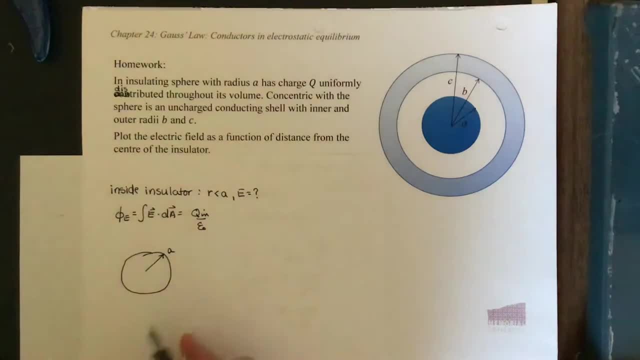 It has radius A, Our Gaussian surface. since we want the electric field inside, let's pick a sphere that's inside. So our Gaussian surface is a sphere with a radius R which is less than this radius A. To start evaluating our answer, we'll need to sort out 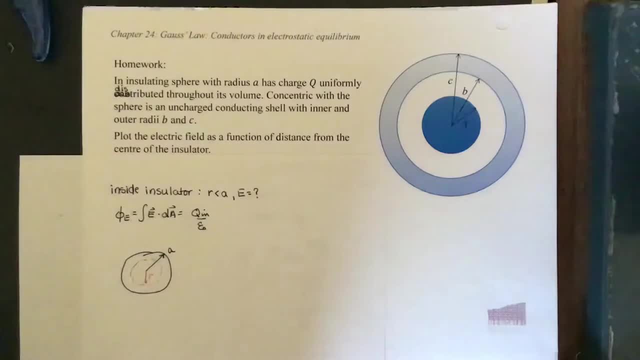 what is the integral of E dot dA? That's a result we're going to use in every single part, so let's do that in general first. Once that's done, we'll be able to come back to it. So if we have spherical symmetry, 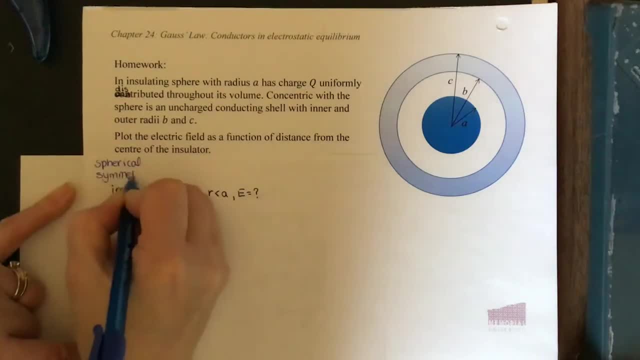 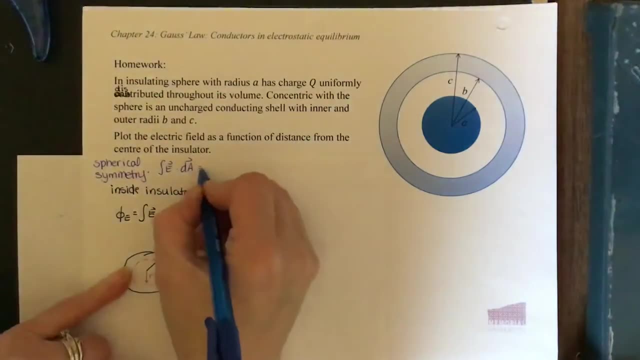 then the integral of E dot dA is equal to the integral of E times dA times cosine of the angle between them. Our electric field points radially outwards and if we look at a little bit of area on that sphere that also points radially outwards. So the angle between those two things is zero. 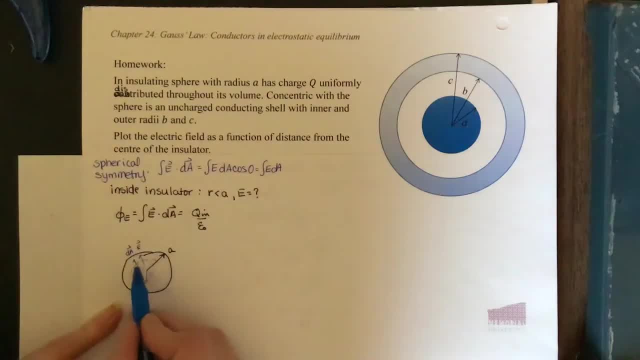 So that's the integral of E times dA. For a constant value of R we'll have a constant value of electric field, so E can come outside our integral dA. the integral of dA is just A. That's the area of our Gaussian surface. 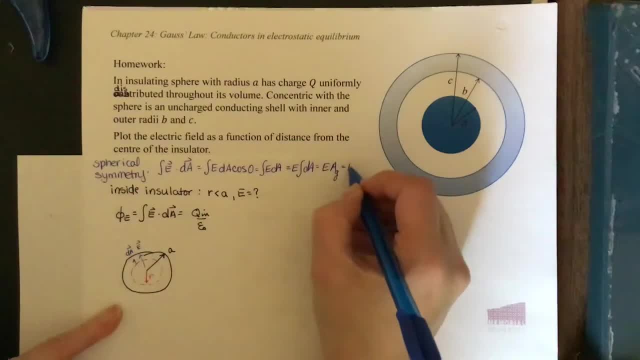 The area of our Gaussian surface is the area of this sphere which is E times 4 pi, R squared. Okay, so we'll use this result for this integral in all of the following steps in the problem as well. So there's the left-hand side of the problem. What about the right-hand side? What is the Q in? Q in means the charge enclosed by the Gaussian surface. If we want to find the charge enclosed by the Gaussian surface, we can do that by putting the Q in find that we know that the charge enclosed would be the charge density rho. times the volume of the Gaussian surface. So what is the charge density? The charge density would be the net charge Q, so the total charge on the sphere divided by the total volume of the sphere. So Q divided by 4 thirds times pi times a. 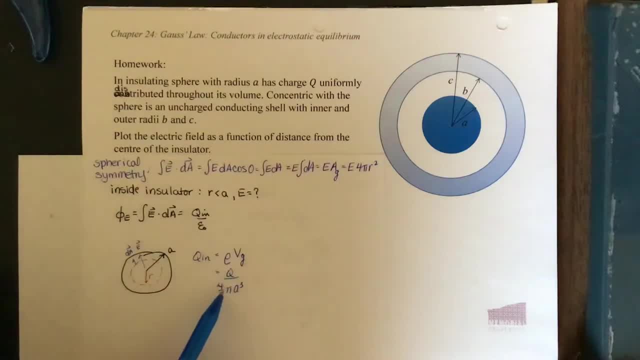 cubed. So our charge density is our total charge divided by our total volume. To find the amount of charge in this Gaussian sphere, we take our charge density and multiply it by the volume of this sphere. 4 thirds pi? r cubed, So that 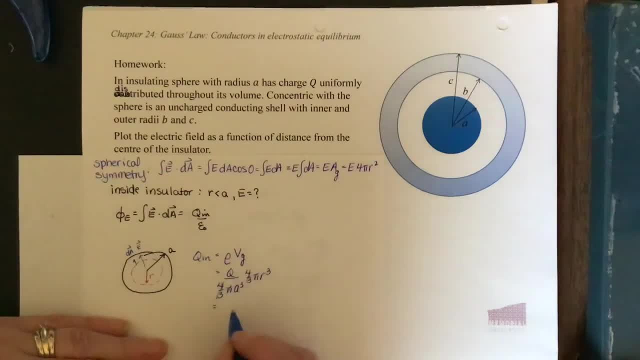 gives us a charge of our 4 thirds pi cancel, so it's the net charge. times r: cubed over a cubed, So the charge inside the sphere is a fraction of the total charge. Let's put these two expressions together. Let's put this in for our.